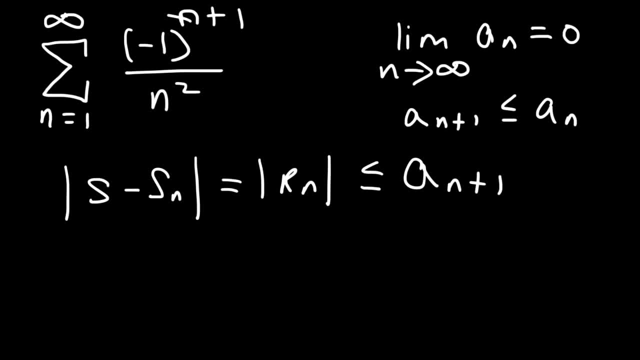 So how can we use this information to approximate this sum correct to two decimal places? First, let's make sure that we have a convergent series. So let's perform the divergence test. As n goes into infinity, what's going to happen to a sub n? Well, we need to know what a sub n is. 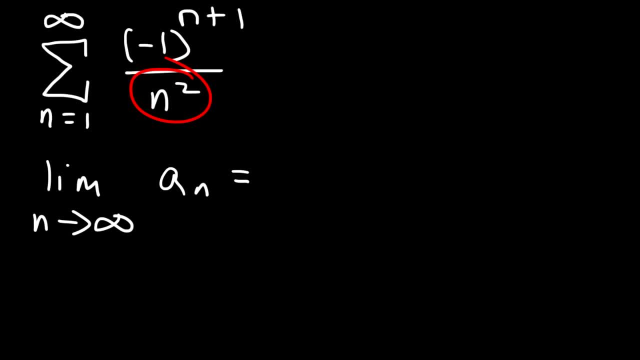 And a sub n is basically 1 over n squared. So the limit, as n goes to infinity, of 1 over n squared that will equal 0.. So it passes the divergence test. Now let's make sure it's a decrease in sequence. So 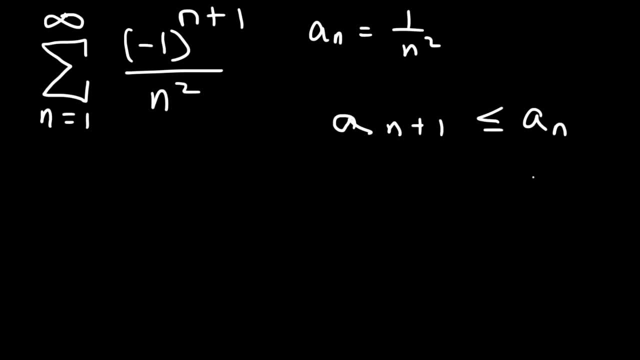 let's show that a sub n plus 1 is less than a sub n. So a sub n is 1 over n squared, which means a sub n plus 1 is less than a sub n. So a sub n is one over n squared, which means a sub n plus 1 is. 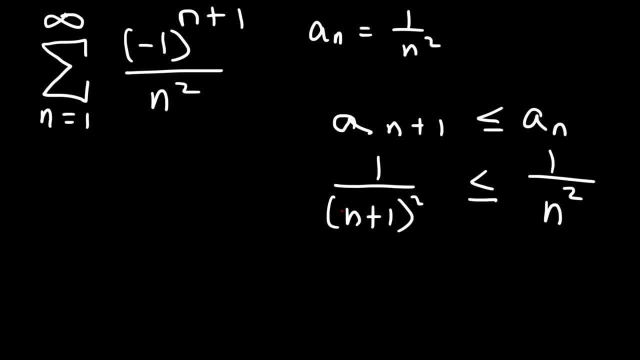 is 1 over n plus 1 squared. Now, because the denominator of this fraction is greater than the denominator of the fraction on the right, this entire fraction is less than that fraction. So therefore we do have a decrease in sequence, which means that the series is convergent. 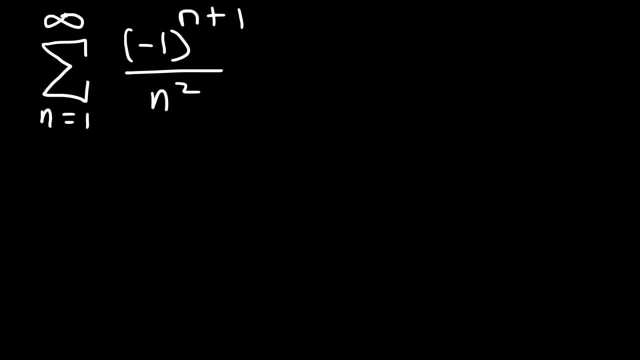 So now that we've established that, we can go ahead and approximate the sum, Now we want it correct to two decimal places. So let's say, if the answer was 5.4312,, for instance, We need this digit to be correct. 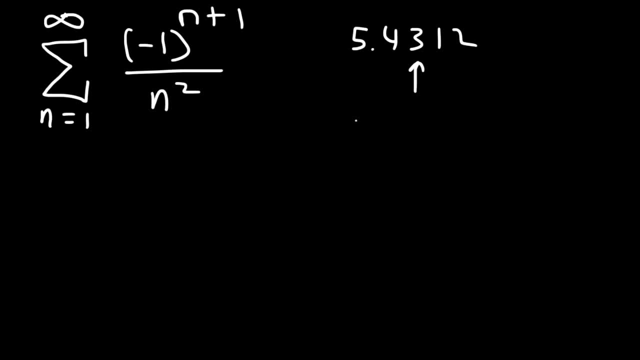 So therefore, just to be on the safe side, you don't want to set your remainder equal to 0.01.. Rather, you want to set it equal to 0.001.. You want this number to be the uncertain digit, but this to be certain. 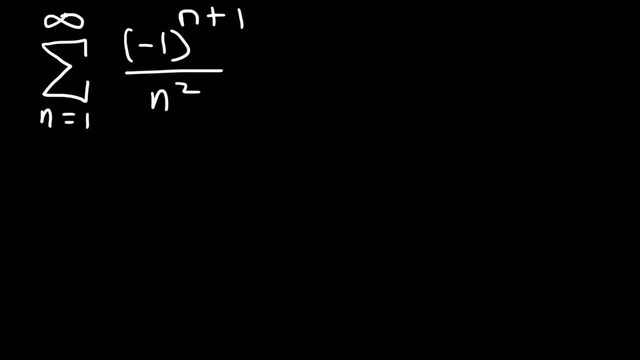 So, in order to approximate the sum, we're going to set the sum to two decimal places. The first thing we need to do is determine how many terms we need, And once we have that, then we can add up those number of terms. 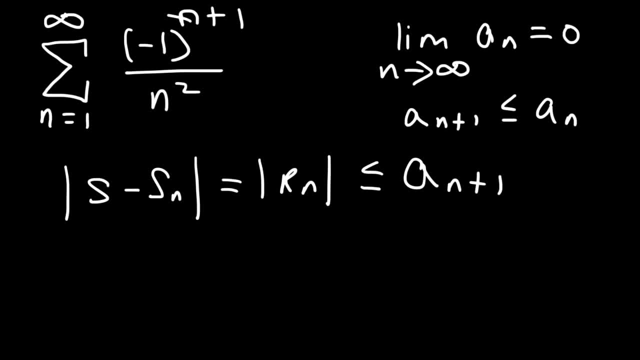 So how can we use this information to approximate this sum correct to two decimal places? First, let's make sure that we have a convergent series. So let's perform the divergence test. As n goes into infinity, what's going to happen to a sub n? Well, we need to know what a sub n is. 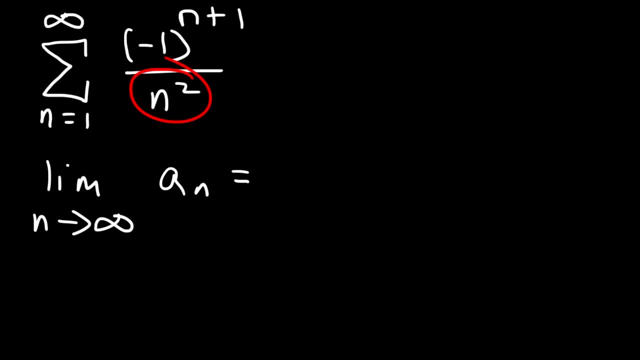 And a sub n is basically 1 over n squared. So let's make sure that a sub n is also 1 over n squared. So the limit as N goes to infinity of 1 over N squared, that will equal 0, so it passes the divergence test. 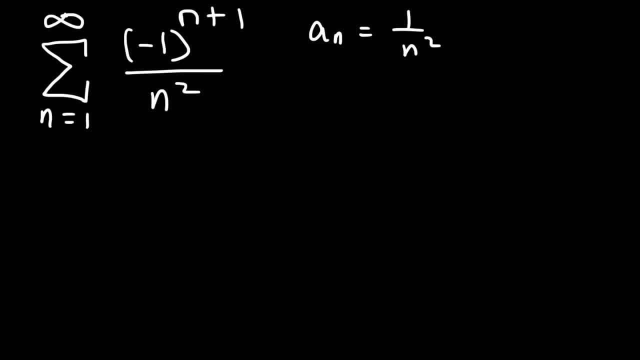 Next we will be looking at A sub n plus 1.. Now let's make sure it's a decrease in sequence. So let's show that a sub N plus 1 is less than a sub N. so a sub n is 1 over n squared, which means a sub N plus 1 is double N squared. 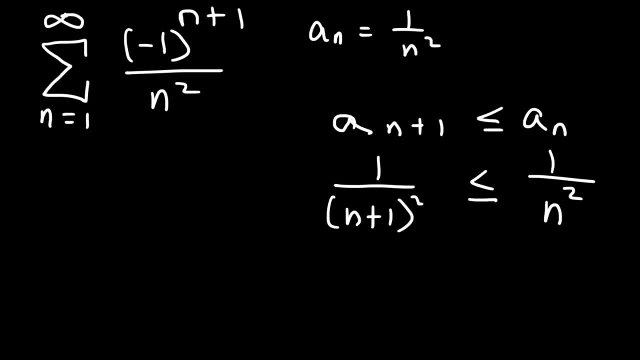 So let's first evaluate this illustration: is 1 over n plus 1 squared. Now, because the denominator of this fraction is greater than the denominator of the fraction on the right, this entire fraction is less than that fraction, So therefore we do have a decrease in sequence. 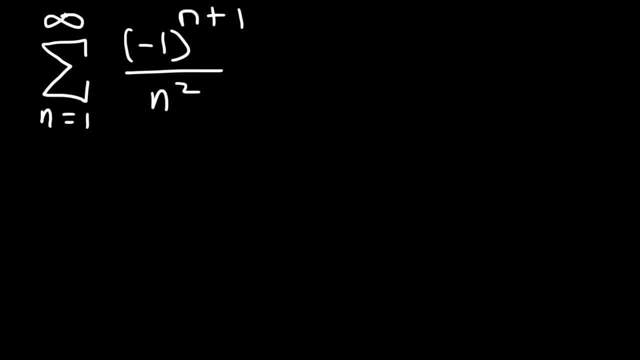 which means that the series is convergent. So now that we've established that, we can go ahead and approximate the sum, Now we want it correct to two decimal places. So let's say, if the answer was 5.4312,, for instance, 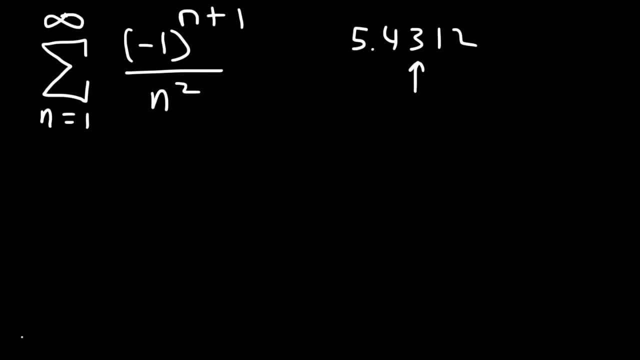 We need this digit to be correct. So therefore, just to be on the safe side, you don't want to set your remainder equal to 0.01.. Rather, you want to set it equal to 0.001.. You want this number to be the uncertain digit. 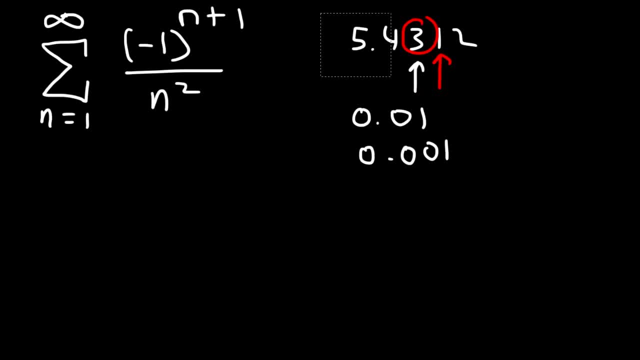 but this to be certain. So, in order to approximate the sum, we're going to set the sum to two decimal places. The first thing we need to do is determine how many terms we need, And once we have that, then we can add up. 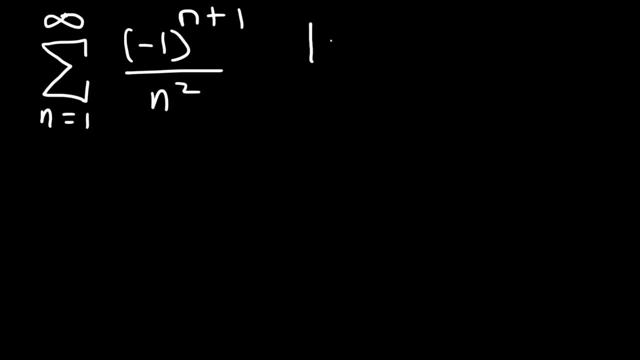 those number of terms. So let's start with this expression: The difference between the infinite sum and the partial sum we set as equal to the remainder which is less than or equal to a sub n plus 1.. Now we're going to focus on this portion of the expression. 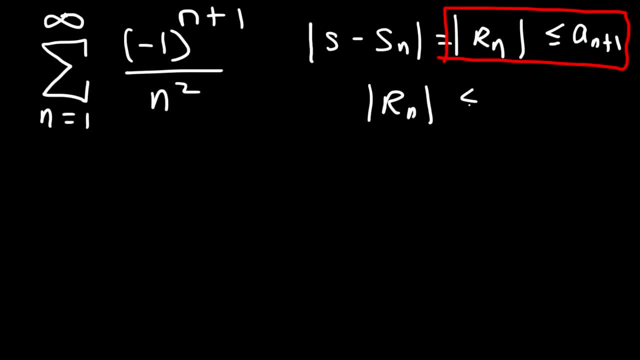 Now a sub n is 1 over n squared, So a sub n plus 1 is going to be 1 over n plus 1 squared. Now we want it accurate to two decimal places, So we want the error to be within 0.001,. 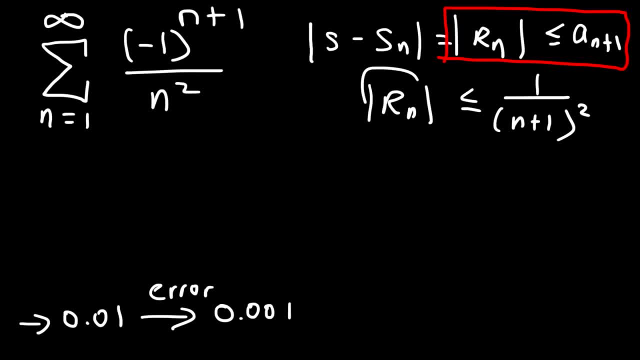 just to be on the safe side. So I'm going to set r sub n equal to 0.001.. And then now let's solve. So I'm going to set r sub n equal to 0.001.. And then now let's solve. 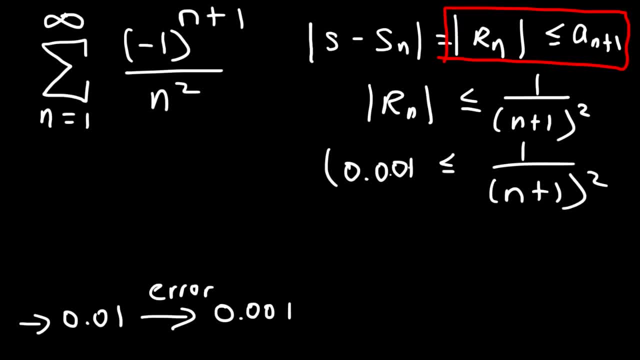 So I'm going to set r sub n equal to 0.001.. And then now let's solve for the value of n. So what we can do is raise both sides to the negative 1 power. 1 divided by 0.001, that's 1,000.. 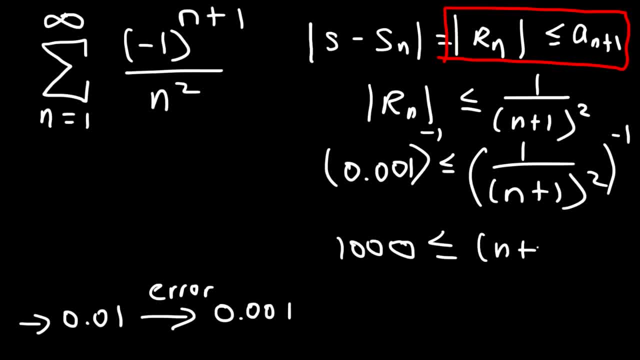 And 1 over n plus 1 squared, that's just going to be n plus 1 squared. Now let's take the square root of both sides. So the square root of 1,000 is about 31.6.. And so that's equal to n plus 1.. 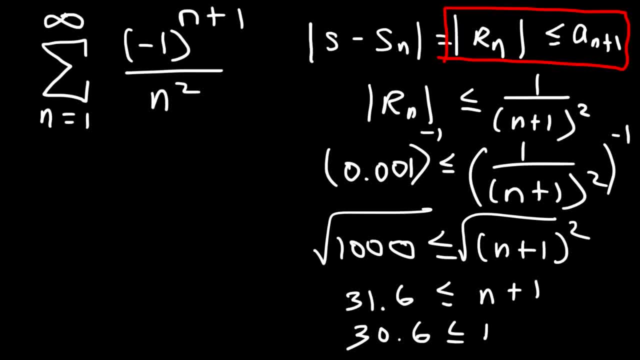 If we subtract both sides by 1,, this is going to be 30.6.. If n is equal to or greater than 30.6,, then we need to say that n is equal to or greater than 31,, because n can only be an integer. 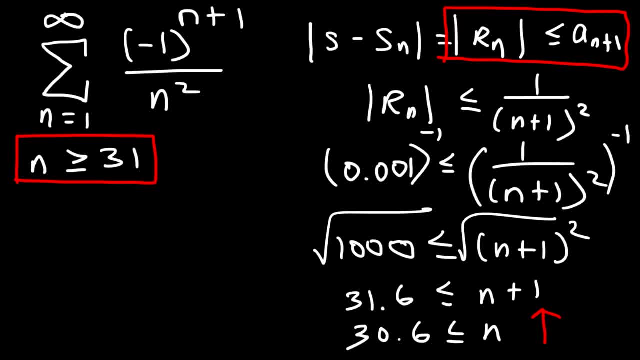 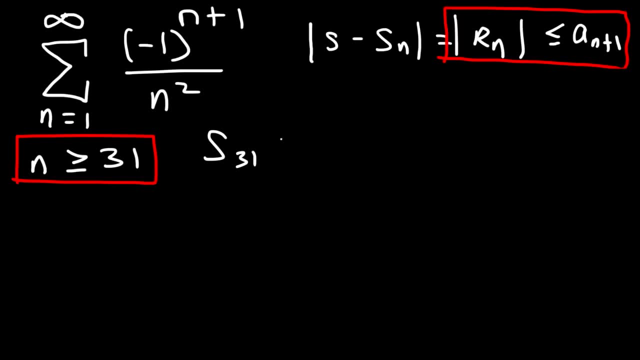 So always round up. So let's go ahead and find the sum of the first 31 terms. Now that's going to take some time, So hopefully you have a calculator where you could just plug this in. So the first term when n is 1, 1 plus 1 is 2.. 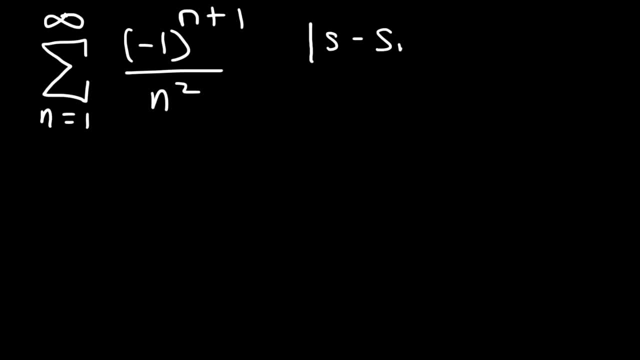 So let's start with this expression: The difference between the infinite sum and the partial sum we set as equal to the remainder, which is less than or equal to a sub n plus 1.. Now we're going to focus on this portion of the expression. 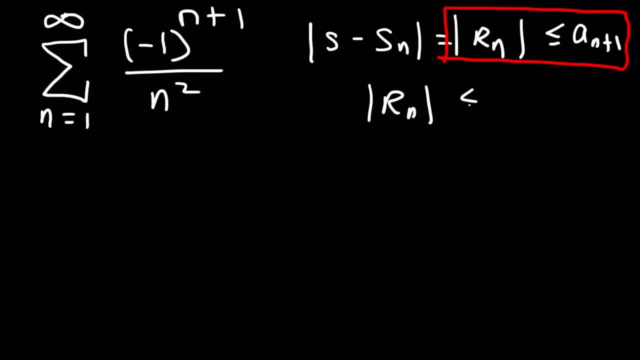 Now a sub n is 1 over n squared, So a sub n plus 1 is going to be 1 over n plus 1 squared. Now we want it accurate to two decimal places, So we want the error to be within 0.001, just to be on the safe side. 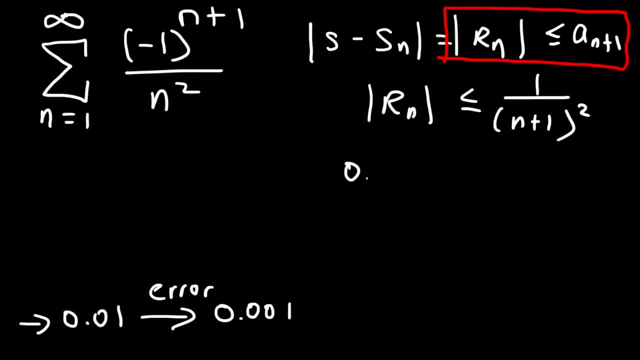 So I'm going to set r sub n equal to 0.001.. And then now let's solve. Let's solve for the value of n. So what we can do is raise both sides to the negative 1 power. 1 divided by 0.001, that's 1,000. 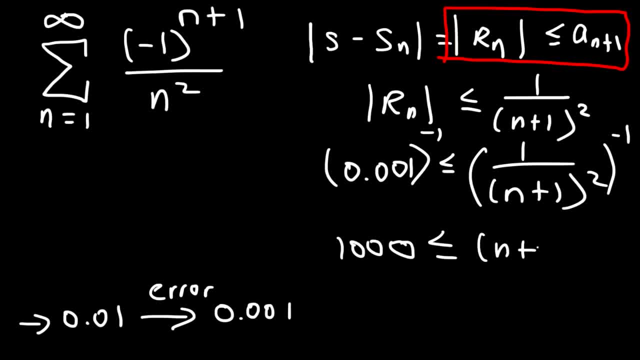 And 1 over n plus 1 squared, that's just going to be n plus 1 squared. Now let's take the square root of both sides. So the square root of 1,000 is about 31.6.. And so that's equal to n plus 1.. 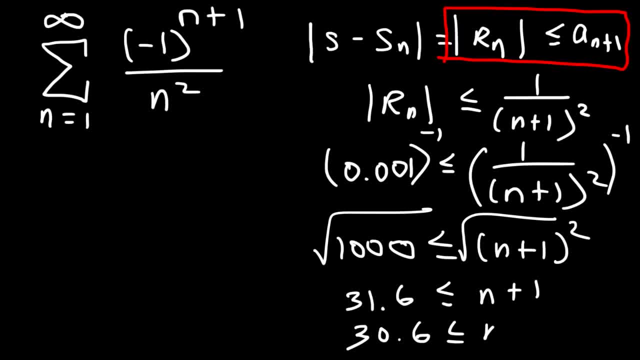 If we subtract both sides by 1,, this is going to be 30.6.. If n is equal to or greater than 30.6,, then we need to say that n is equal to or greater than 31,, because n can only be an integer. 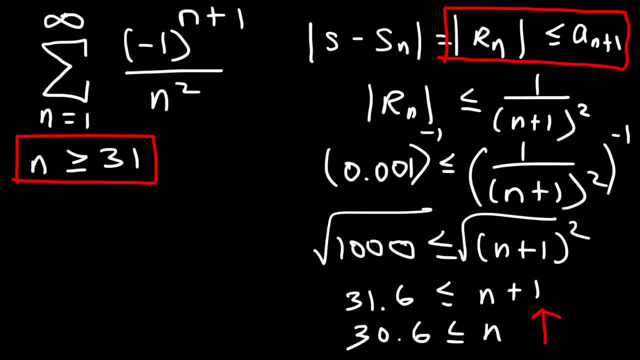 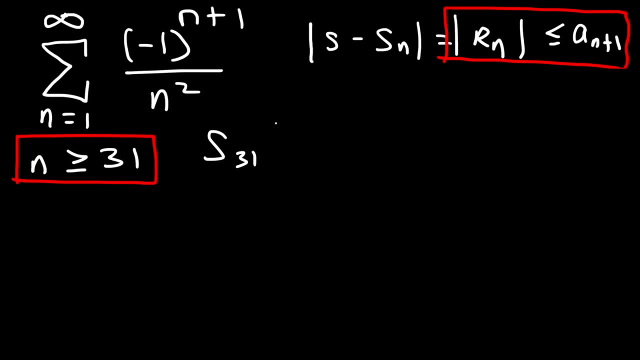 So always round up. So let's go ahead and find the sum of the first 31 terms. Now that's going to take some time, So hopefully you have a calculator where you could just plug this in. So the first term when n is 1, 1 plus 1 is 2, negative 1 squared is positive 1.. 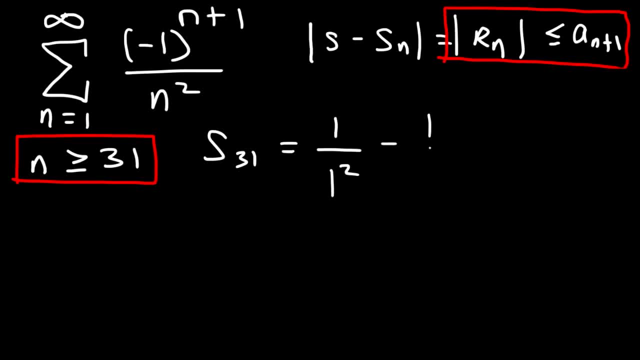 So it's going to be 1 over 1 squared, Then the next one is going to be 1 over 2 squared. So the next term is going to be 1 over 2 squared, And then the next term is going to be 1 over 1 squared. 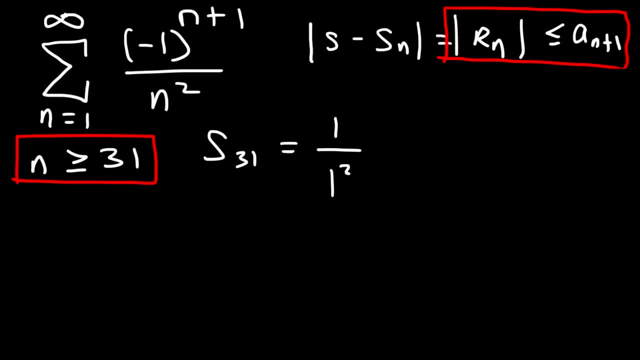 Negative 1 squared is positive 1.. So it's going to be 1 over 1 squared. The next one is going to be 1 over 2 squared And then plus 1 over 3 squared And then minus 1 over 4 squared. 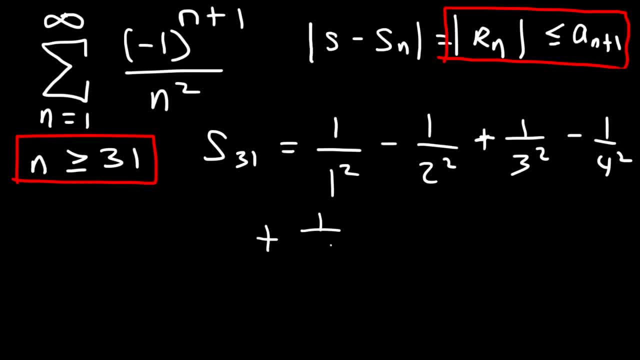 And then it's going to be plus 1 over 29 squared if you continue it, And then minus 1 over 30 squared, plus 1 over 31 squared. Now go ahead and plug that into your calculator. If you do, you'll get that the sum of the first 31 terms is 0.822.. 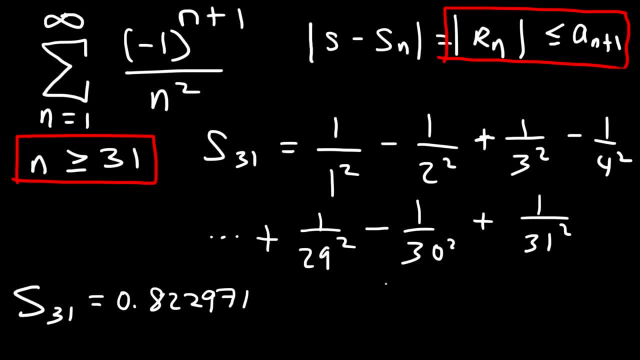 Now, just to be on the safe side, go ahead and plug in 100 as well. The sum of the first 100 terms is going to be 0.8224175.. So in both cases the sum rounds to 0.82.. 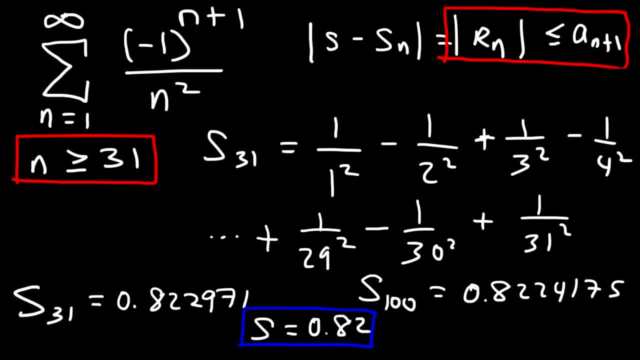 So, if you want to round it correct to two decimal places, set your error equal to 0.001.. And you'll be on the safe side if you do that. Now what happens if we set our error to 0.01?? Well, let's say if, since we already set the error to 0.001,, 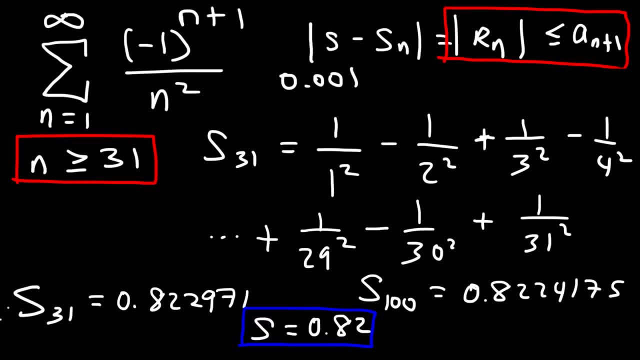 let's say, if we wanted the answer correct to three decimal places, And let's say we chose this error. For me personally, if I want the answer correct to three decimal places, I would choose an error of something less 0.0001. 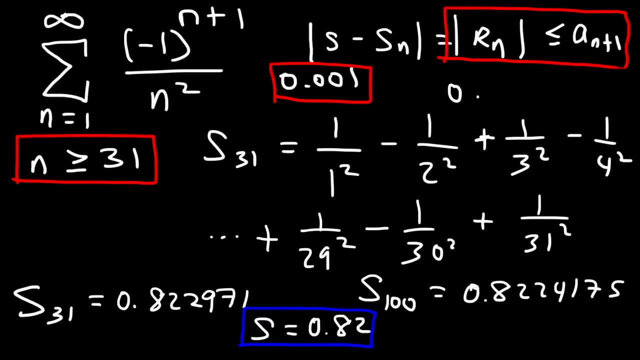 And it usually works out in my case when I do that. But let's say, if we want to round it to three decimal places and we set the error to 0.001.. In this case, n will still be the same because we used 0.001 in this example. 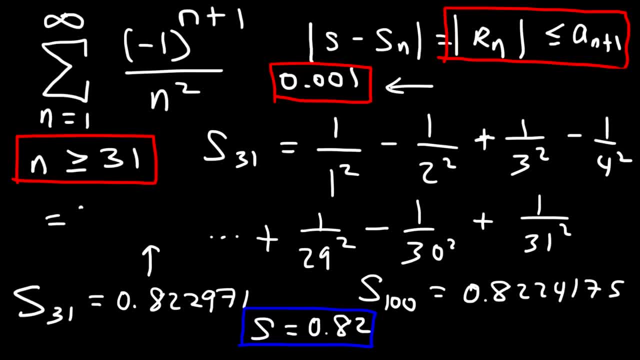 But rounding this number to three decimal places, it's going to be 0.823.. And rounding this one to three decimal places is 0.822.. But these answers are not the same. So if you want to round it to three decimal places, 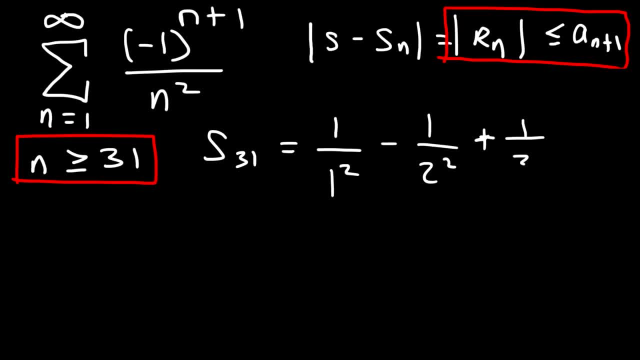 And then plus 1 over 3 squared, and then minus 1 over 4 squared, And then it's going to be plus 1 over 29 squared if you continue it, And then minus 1 over 30 squared, plus 1 over 31 squared. 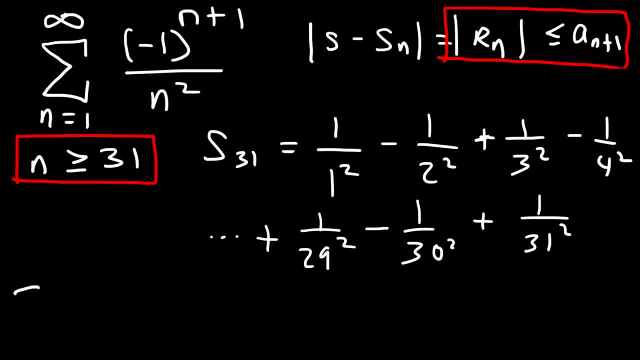 Now go ahead and plug that into your calculator. If you do, you'll get that the sum of the first 31 terms is 0.822971.. Now, just to be on the safe side, go ahead and plug in 100 as well. 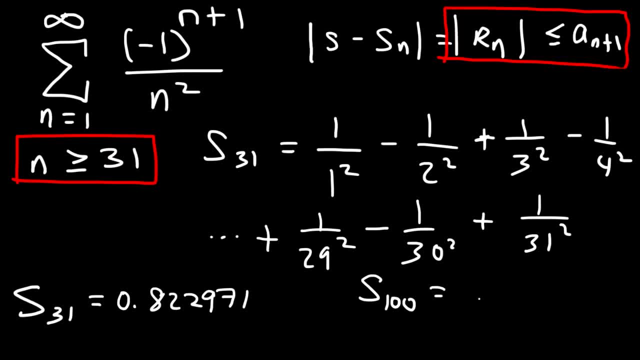 The sum of the first 100 terms is going to be 0.8224175.. So in both cases the sum rounds to 0.8224175.. So if you want to round it correct to two decimal places, set your error equal to 0.001. 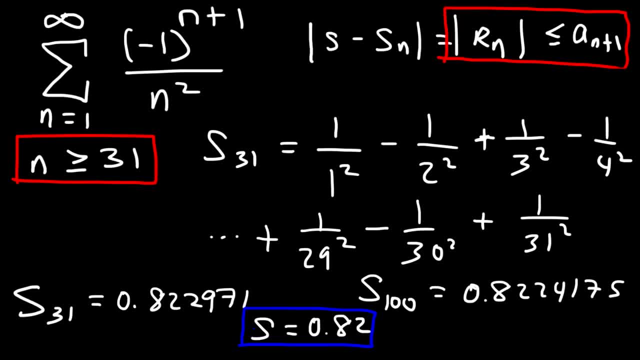 And you'll be on the safe side if you do that. Now, what happens if we set our error to 0.01?? Well, let's say if, since we already set the error to 0.001,. let's say if we wanted the answer correct to three decimal places. 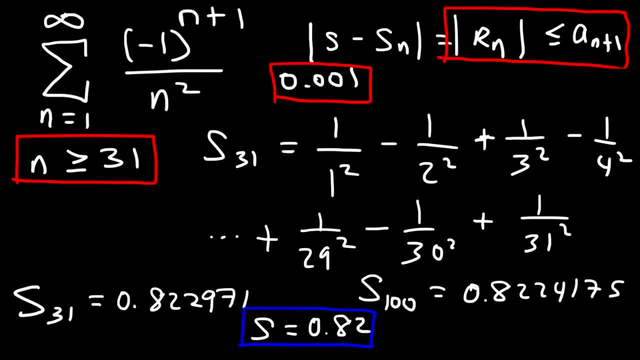 And let's say we tried to round it to 0.001.. And we chose this error. For me personally, if I want the answer correct to three decimal places, I would choose an error of something less 0.0001.. 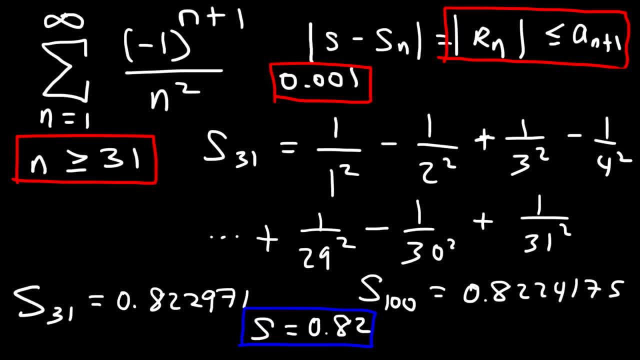 And it usually works out in my case when I do that. But let's say, if we want to round it to three decimal places and we set the error to 0.001.. In this case, n will still be the same because we used 0.001 in this example. 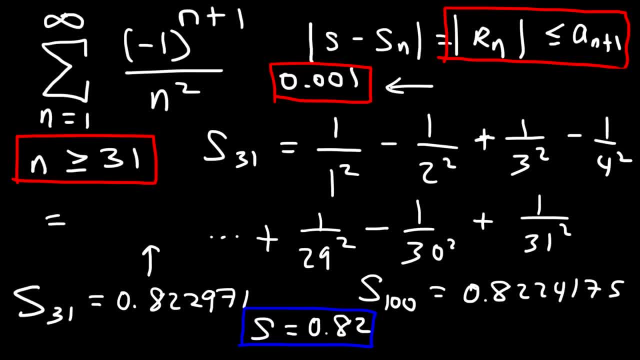 But rounding this number to three decimal places, it's going to be 0.0001.. And rounding this one to three decimal places, it's going to be 0.822.. So notice that these answers are not the same. So if you want to round it to three decimal places, 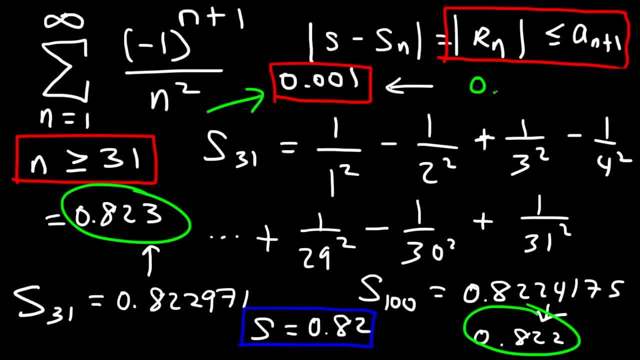 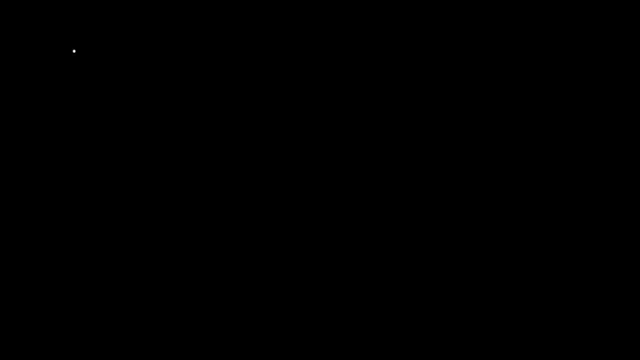 I recommend not choosing this as an error, but choose something less, Ten times less, 0.0001.. And you'll be on the safe side if you do it that way. So let's try a similar problem, But it's going to be a little different from the previous one. 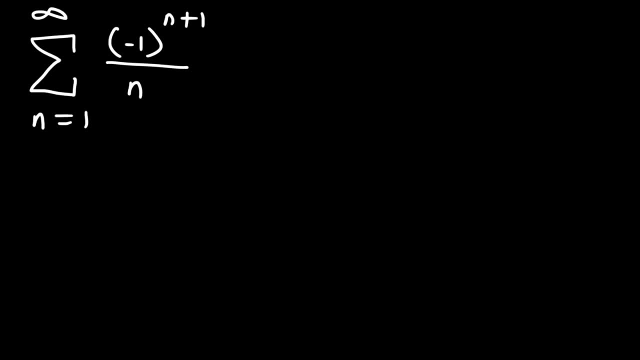 Everything is going to be the same. But instead of dividing by n squared, we're going to divide it by n cubed. So 1 over n squared, 1 over n squared, 1 over n cubed: It passes the divergence test. 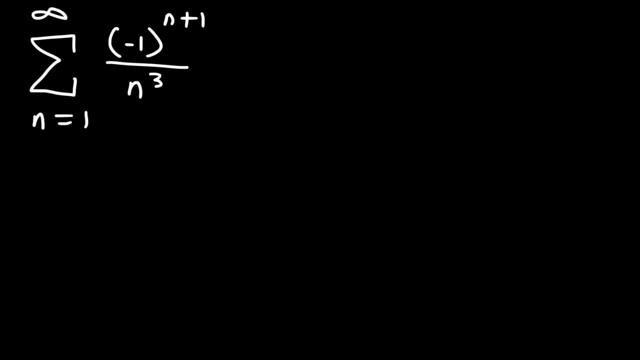 Because 1 over n? squared also passed the divergence test And at the same time 1 over n cubed is a decrease in function, Just as 1 over n? squared is a decrease in function. So we don't have to show that those conditions are met. 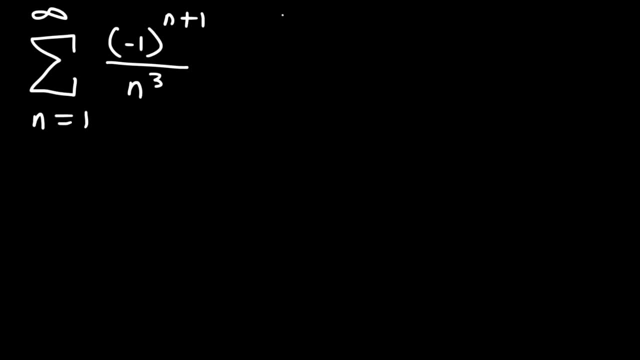 Now let's approximate the sum correct to three decimal places. Feel free to pause the video and try this problem. So we want this last digit to be accurate. So therefore I'm going to set my error to four decimal places. So let's start with this. 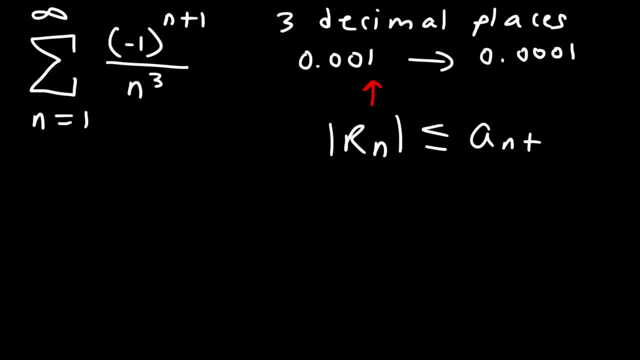 r sub n, Let's set it equal to a sub n plus 1.. So the error is 0.0001.. Now my a sub n is 1 over n cubed, So a sub n plus 1.. That's 1 over n plus 1 cubed. 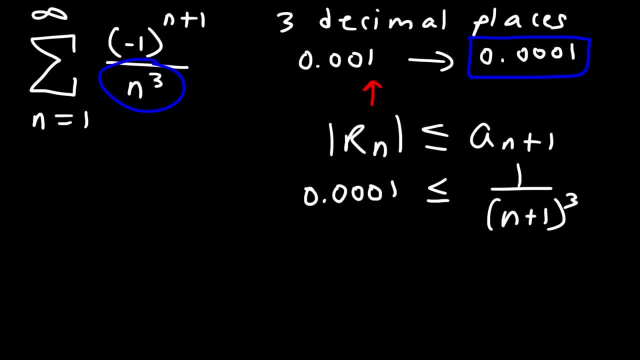 So let's determine how many terms we need in order for the answer to be accurate to three decimal places. So let's raise both sides to the negative 1 power, So 1 divided by 0.0001.. That's 10,000.. 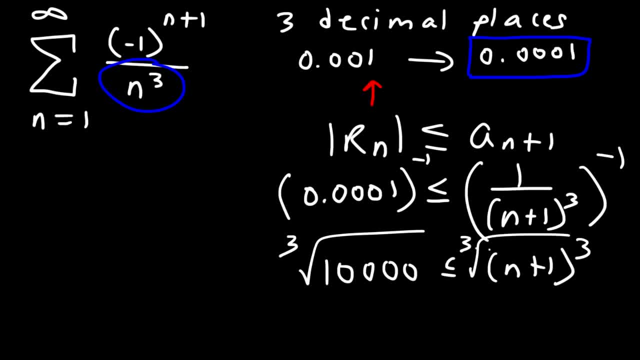 Now what we need to do is take the cube root of both sides, So the cube root of 10,000.. Or 10,000 raised to the 1 third, That's 10,000.. That's 21.5.. 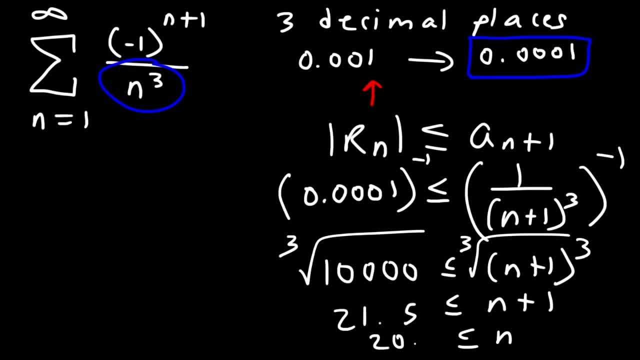 So that's equal to n plus 1.. Subtracting both sides by 1, we're going to get 20.5.. So we need to round it up. So therefore, n has to be equal to or greater than 21 if we want the answer to be accurate. 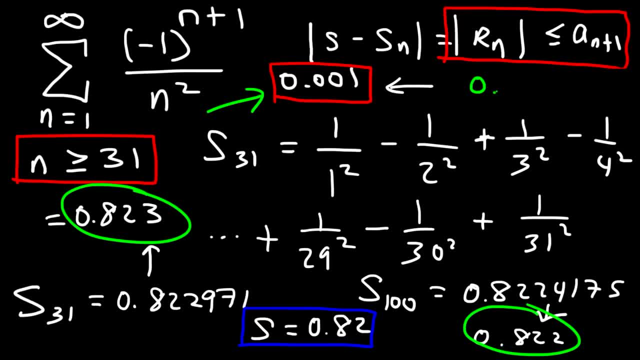 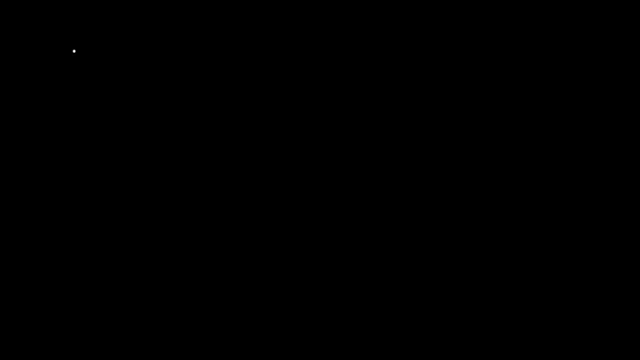 I recommend not choosing this as an error, but choose something less, 10 times less, 0.0001.. And you'll be on the safe side if you do it that way. So let's try a similar problem, but it's going to be a little different. 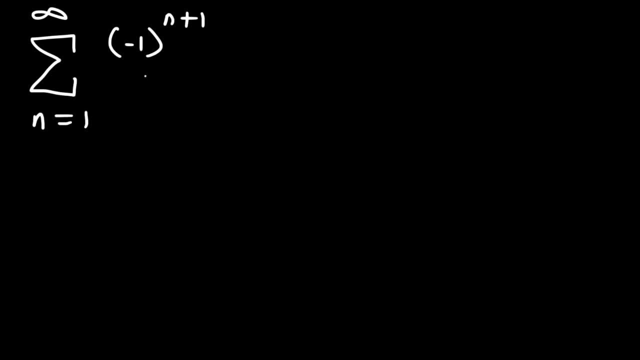 from the previous one. Everything is going to be the same, but instead of dividing by n squared, we're going to divide it by n cubed. So 1 over n cubed it passes the divergence test, because 1 over n squared also passed the divergence test. 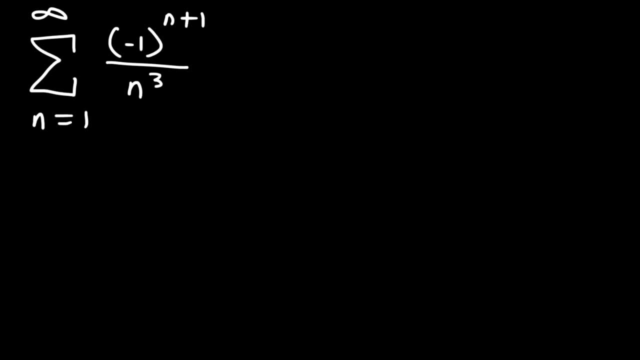 And at the same time, 1 over n cubed is a decrease in function, just as 1 over n squared is a decrease in function. So we don't have to show that those conditions are met. Now let's approximate the sum. 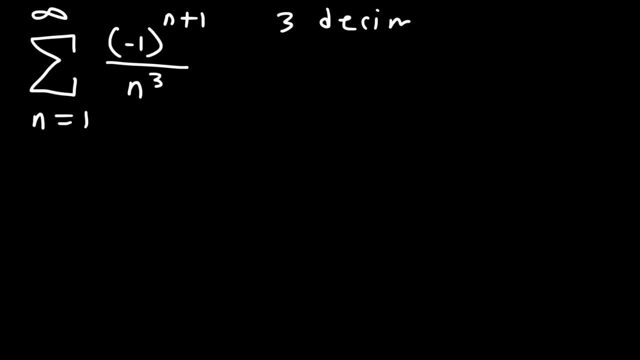 Correct to three decimal places. Feel free to pause the video and try this problem. So we want this last digit to be accurate, So therefore I'm going to set my error to four decimal places. So let's start with this r sub n. let's set it equal to a sub n plus 1.. 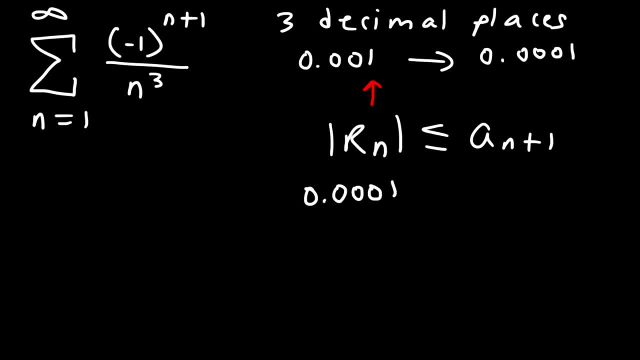 So the error is 0.0001.. Now my a sub n is 1 over n cubed, So a sub n plus 1, that's 1 over n plus 1 cubed. So let's determine how many terms we need. 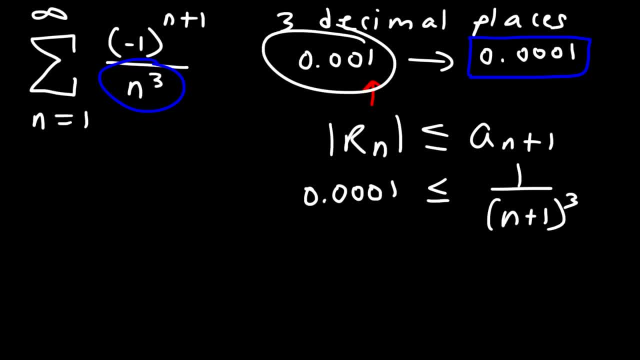 in order for the answer to be accurate to three decimal places. So let's raise both sides to the negative 1 power. So 1 divided by 0.0001, that's 10,000.. Now what we need to do is take the cube. 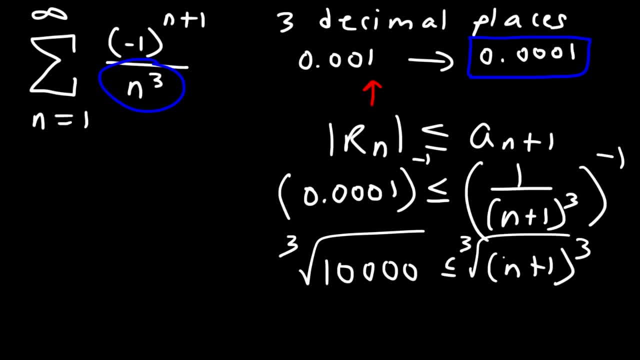 the cube root of both sides. So the cube root of 10,000, or 10,000 raised to the 1 third, that's 21.5.. So that's equal to n plus 1.. Subtracting both sides by 1, we're going to get 20.5.. 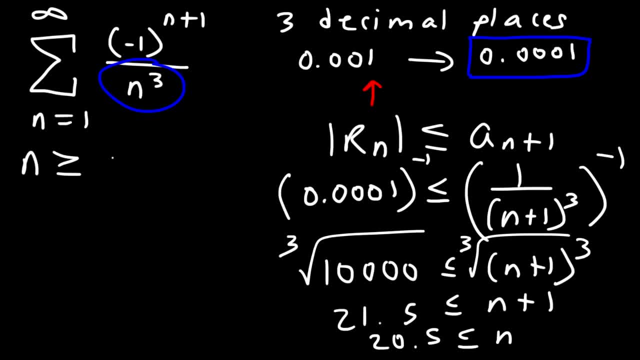 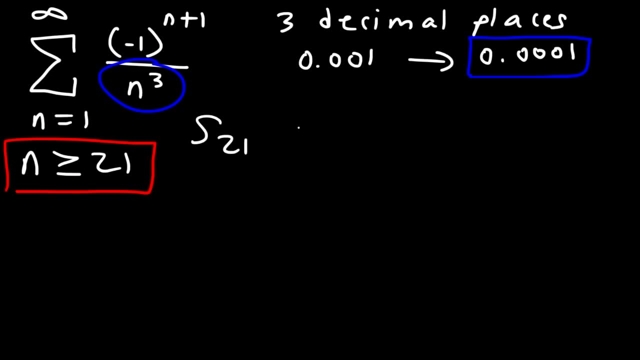 So we need to round it up. So therefore, n has to be equal to or greater than 21 if we want the answer to be accurate within three decimal places. So let's calculate the sum of the first 21 terms. So if we plug in 1, the first term is going to be positive. 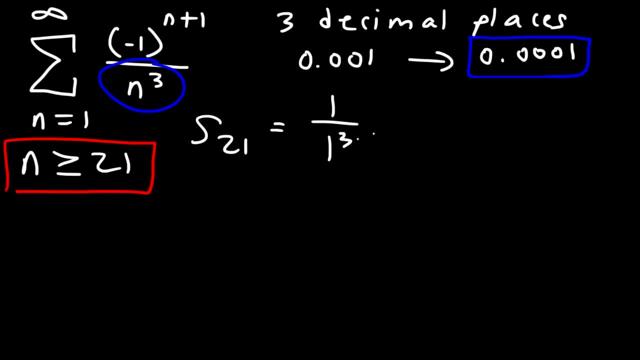 Negative, 1 squared is positive. So it's 1 over 1 cubed minus 1 over 2 cubed, and then plus 1 over 3 cubed minus 1 over 4 cubed. Now all of the even ones are negative. 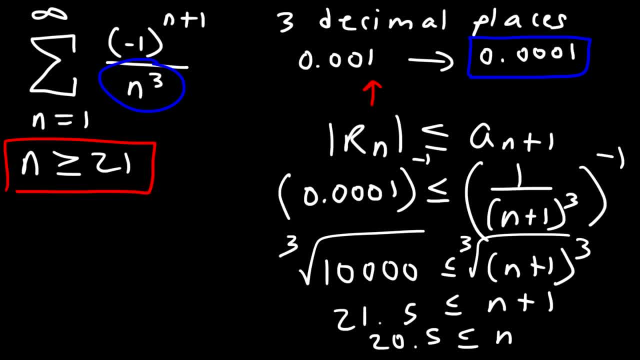 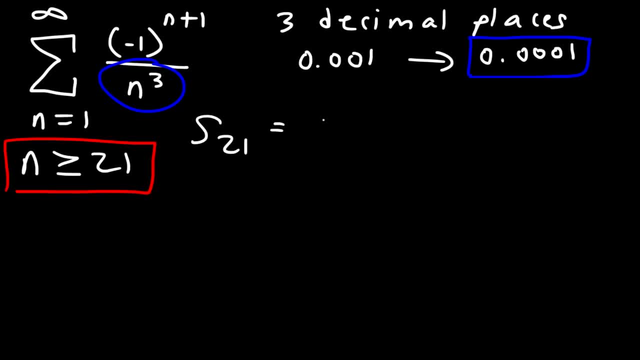 within three decimal places. So let's calculate the sum of the first 21 terms. So if we plug in 1, the first term is going to be positive, Negative. 1 squared is positive, So it's 1 over 1 cubed minus 1 over 2 cubed. 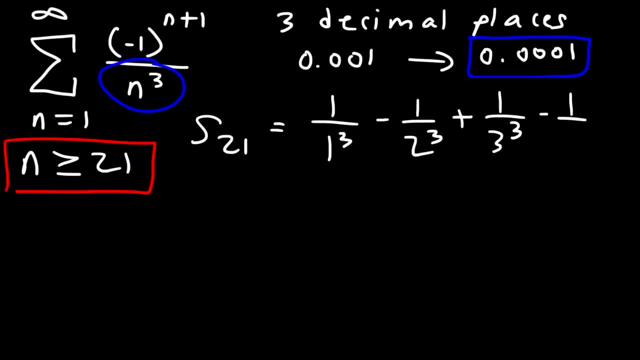 And then plus 1 over 3 cubed, minus 1 over 4 cubed, Now all of the even ones are negative and all of the odd ones are positive. So the last term is an odd term, So it's going to be a positive one. 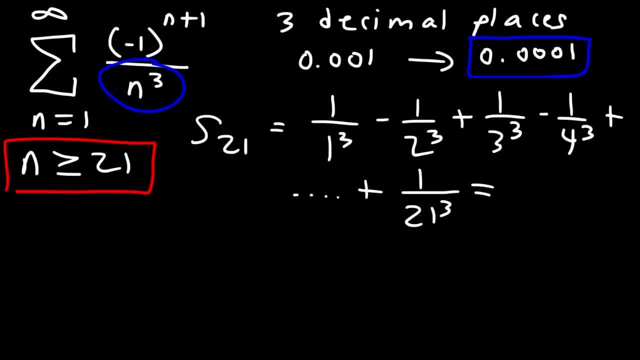 This is going to be plus 1 over 21 cubed, So go ahead and plug that in and see what answer you get. So you should get 0.901593.. So therefore, rounded it to three decimal places, we can say that s is approximately. 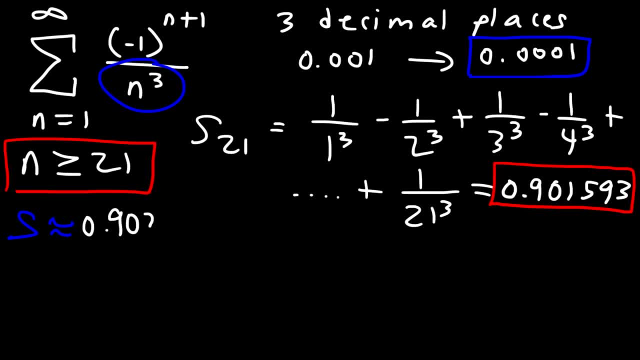 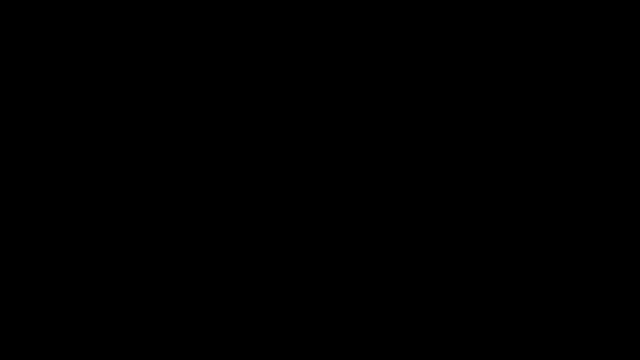 0.902.. And then if we plug in 1 over 2 cubed minus 1 over 2 cubed, we get 1 over 2 cubed. 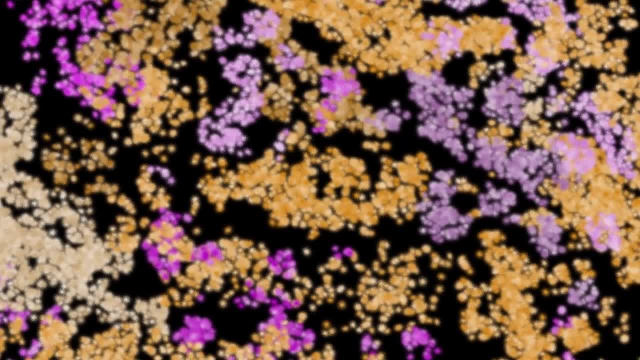 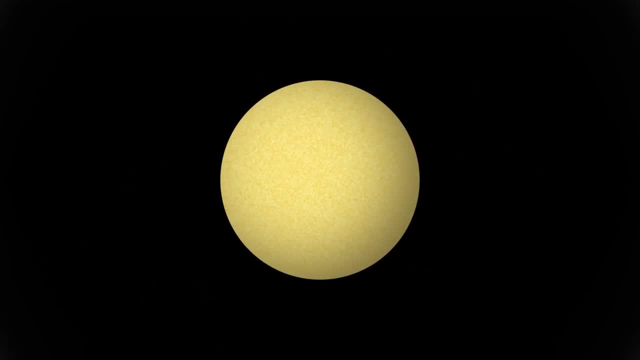 The universe is made of matter. 98% of this matter- ignoring the dark matter- is pure hydrogen and helium, But thankfully, billions of years ago, supergiant stars fused the hydrogen and helium into all the other elements and then exploded them all over the 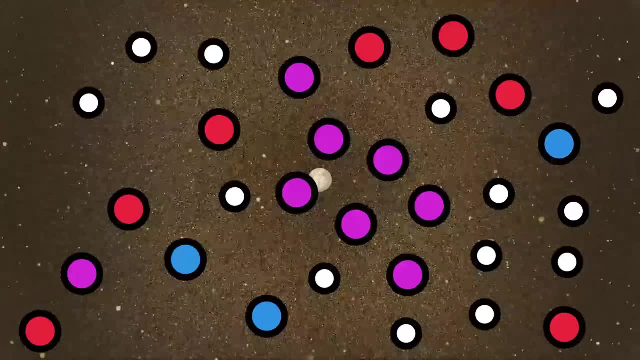 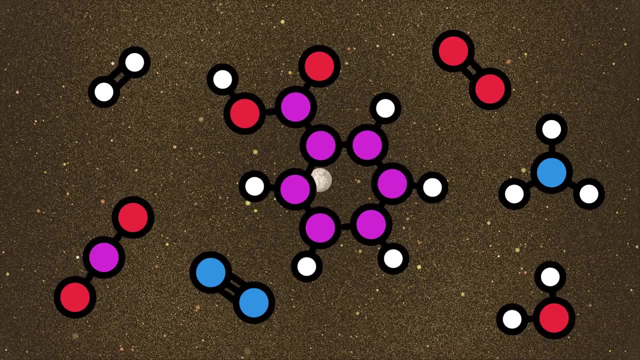 universe, And that's where chemistry came from. These elements grouped together into a vast array of different molecules, and these molecules combined with each other in a stupendous number of complicated ways. Chemistry is the subject that studies this matter in all its forms, and